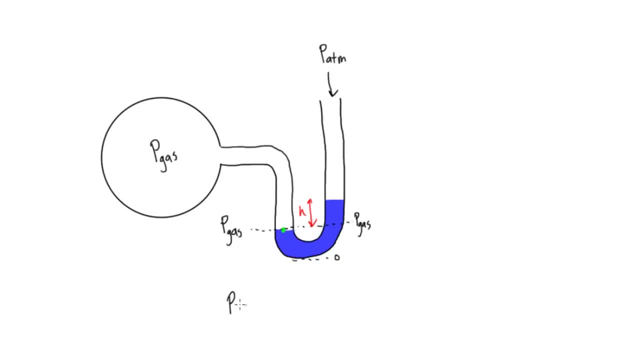 regular equation here We have: P is equal to. so P that we want is equal to P that we're given, you know, plus or minus rho GH. Now we're looking at this and this pressure here is obviously going to have to be less than this pressure here, because as you go, as you increase depth, or as 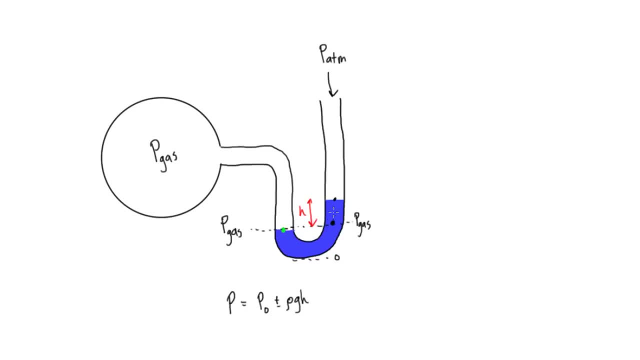 you go deeper into a fluid, the pressure increases, right, Because you have all of that weight of fluid on top of you as well. So in this case, because we're going up, we're going to have to subtract. So, just visually, we're going to have to know that this is definitely going to be a 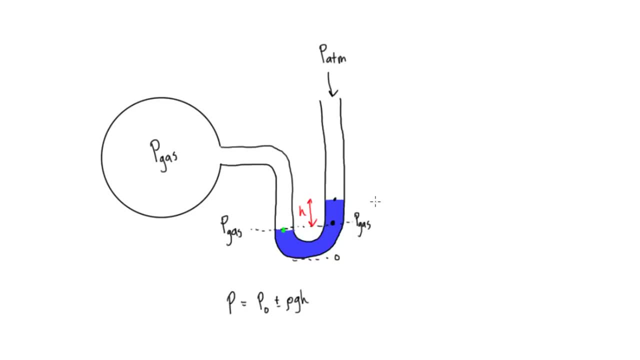 less pressure. So we're going to call this pressure right here, this pressure which is equal to P-atm. So then we're going to say that P-atmosphere is equal to- well, P-gas. In this case it is minus. 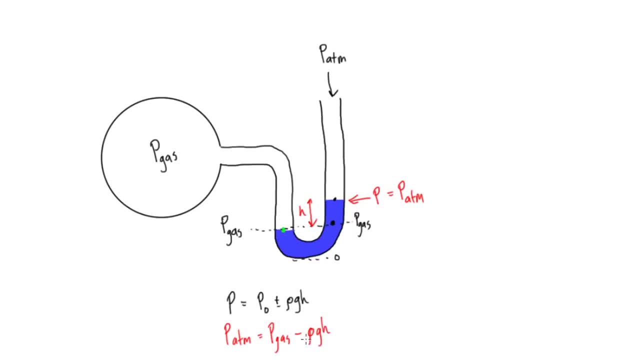 rho, GH And rho is the density of whatever fluid we're using. So we could be using water or we could be using mercury. Just make sure you know what the density is at the given temperature. Something else to consider is what if we have here- I'm going to try and copy this: 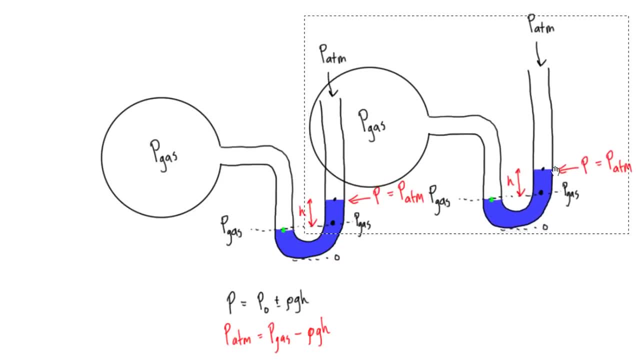 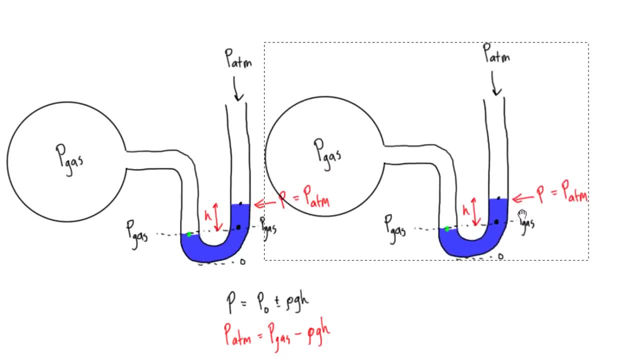 Let's see if we have space to put it aside. We're going to run out of space. You know what? Here I got this. It's okay, There we go, All right. So what if we have another setup? Maybe let's go in and just erase some of this. 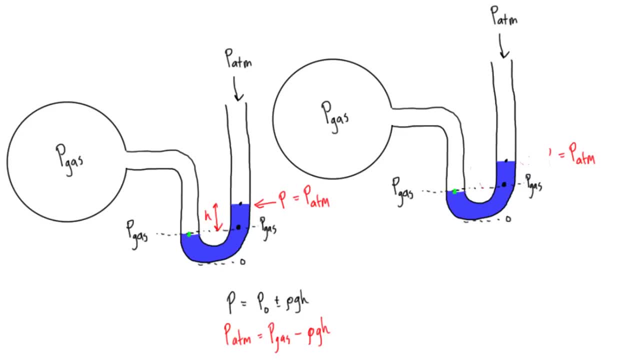 stuff. Actually, that's fine. We can leave that. Basically, what I want to say is: what if we have the fluid? what if we have the level, like this: Okay, All right. So now what we're saying is the surface that's in contact with the gas is going to be higher than the 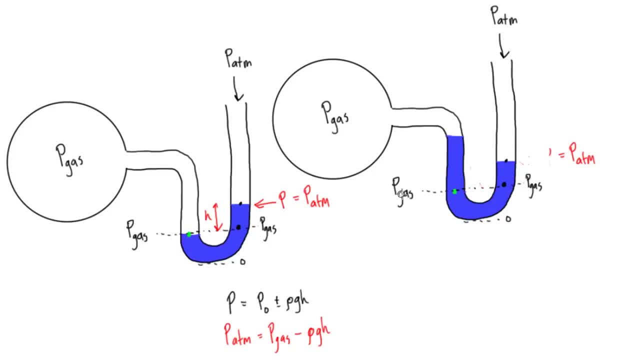 surface that's in contact with the atmosphere. Well, again, we can just maybe get rid of some of this distracting stuff. Yeah, Sorry about that. All right, That's good enough. Maybe we'll get rid of some of these dotted lines. Okay, So I hope you're still with. 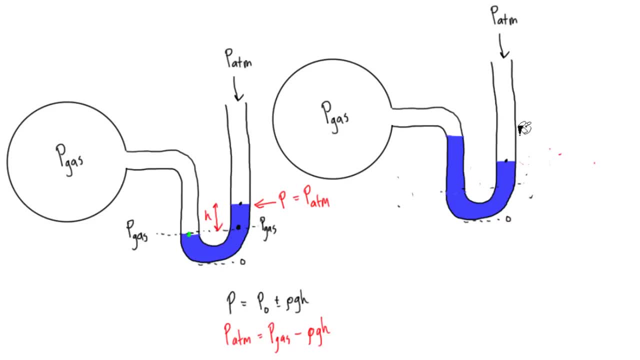 me here. We'll fill in those. It's a brand new manometer. It's like it's never been used before. All right, So what we're going to do is we're going to say that now this level right here that we're looking at this level has the pressure of P gas right? It's in contact with this gas. 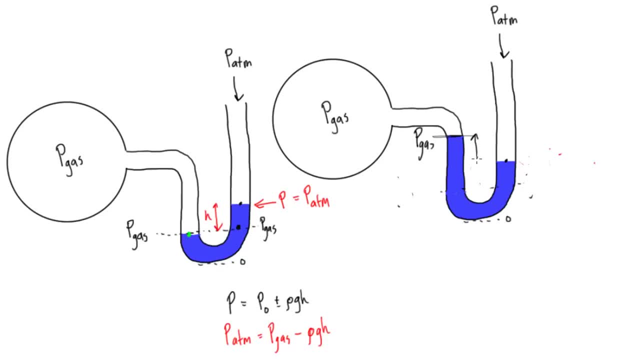 So it's pressing down The fluid here. And then we're looking at, this is going to be our difference in height in the water column, And then, right here, this is going to be P atmosphere. right, P atmosphere is pushing down on this water right there. So we use our regular formula, So we have pressure that we want. 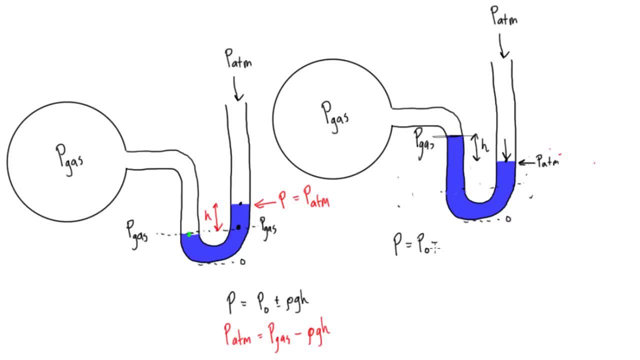 is equal to the pressure that we're given: P naught plus or minus rho G, H. Now, this is the way that I like to solve them, And so I just have this plus or minus here. Now we're going down. So this, this level right here, is also okay. So we have this height above zero and we also have 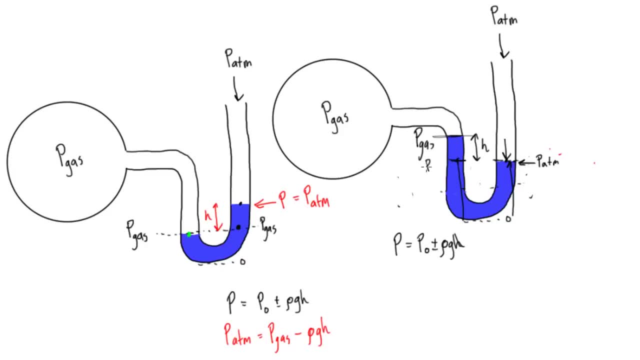 the same height above zero right here. So we're also going to have P atmosphere anyway. So what we're saying is: we have pressure gas here, We're going to increase our depth, We're going to go deeper into this fluids. The pressure has to increase. So P atmosphere must be P gas plus. 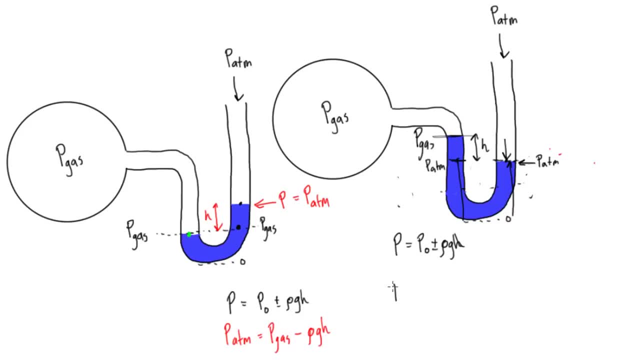 some positive term. So we can say that we're looking for P P T M is equal to P gas plus rho G H. Rho G H- Again rho- density of whatever fluid we're working with, usually water and mercury, or sometimes oil, things like that. So yeah, here we go, That's how. 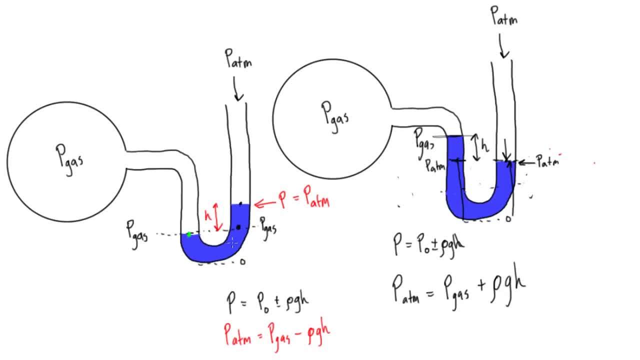 we solve a simple manometer problem. We call it simple if there's one fluid and we can put more fluids in it and we'll call that a compound manometer. but we'll get to that later. So I think next video I'll go over an example with some actual manometers. 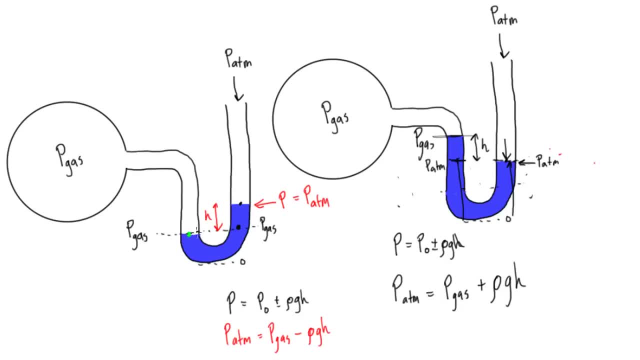 But this is the general idea. You want to make sure, you want to figure out which side of the water is higher, if it's the atmospheric side or the gas side, and then you add or subtract correspondingly this rho, G, H term. And just to hit that point home, just imagine if you have 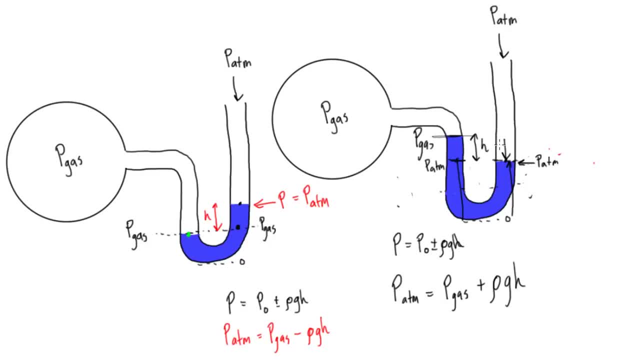 this tube that's a uniform diameter everywhere, and you have this pressure pushing down here that's forcing the liquid up. Well then, this pressure would have to be greater than this pressure. right? It's just a simple force balance. Same on this one. If this pressure is pushing down harder,